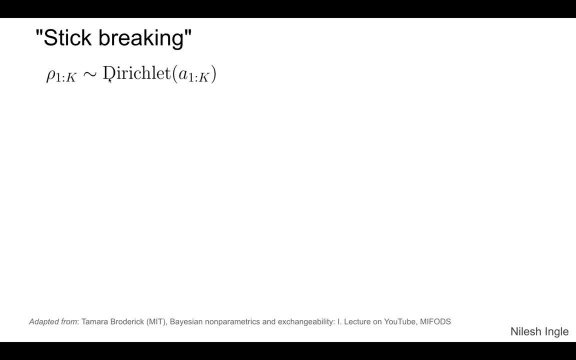 and here, what we have up here is first to draw the probability row for each of the classes. We can use the distribution where the parameters import would be each separate hyper parameter for each separate class, k and in the stick breaking process, which we'll talk in just a moment, We would be using 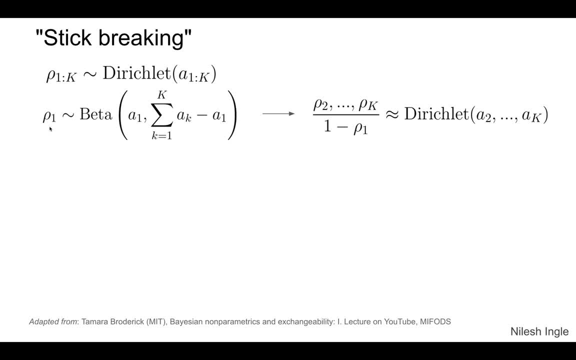 beta distribution to draw the value for row 1 and then use the Dirichlet distribution to draw values on the remaining set for rows. So this does not have k1 in this particular input hyper parameters. So the idea is like this and I'll try to explain it in a less confusing way if I can. 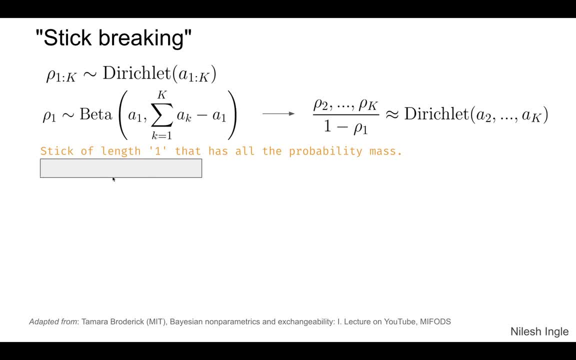 I hope I am able to do that. Let's imagine a stick of length 1, so that would be a total probability mass that we have. Now what we are going to do is we'll break a part of the stick, So we'll have the probability mass. 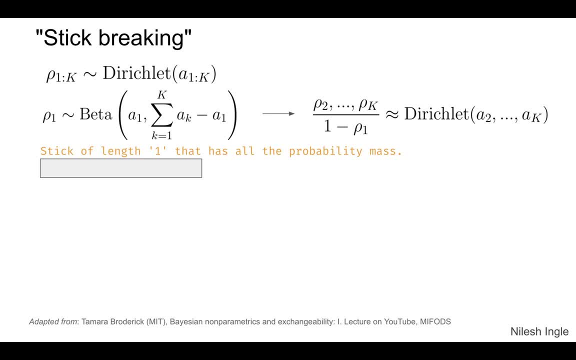 coming off from the stick and part of it that remains on the stick. So the very first part we broke off. let's say we broke off part v1.. so the beta proportion then for that part v1 we would be getting from a beta distribution. 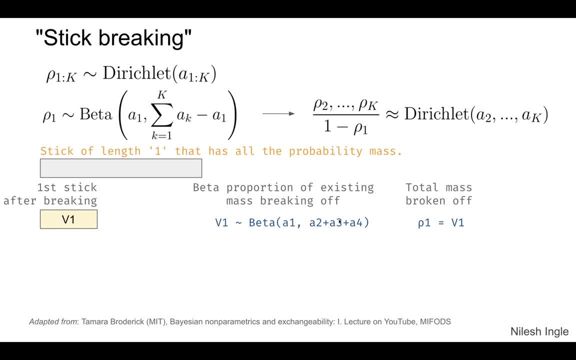 where the input parameters would be a1 and a2 plus a3 plus a4, as shown up here. so we are subtracting a1 and therefore we do not have a1, because- and we are using that here. so the total mass broken off is rho1 is equal to v1 that we get from this beta distribution. 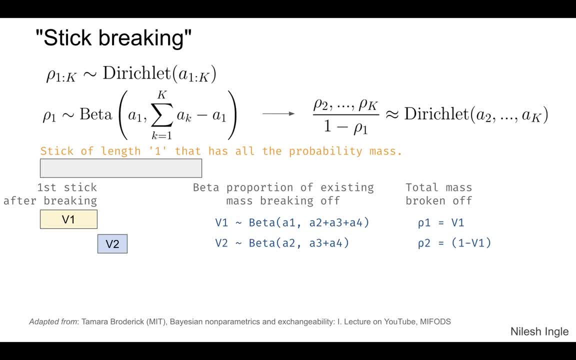 next what we do is, whatever is remaining, we break off another piece, v2, and again in this case the hyper parameters for beta now are a2 and a3 plus a4 and you. the total mass broken off then is 1 minus v1, and so on for v3, and finally we are left with v4. 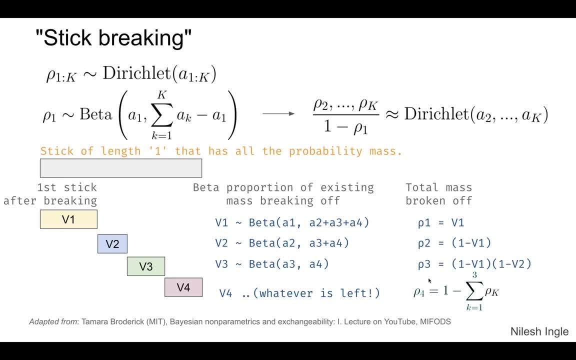 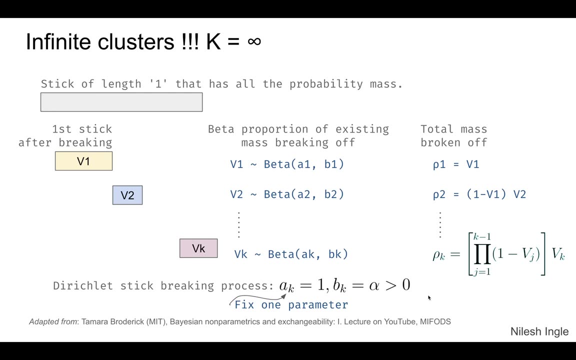 and we. this is the notation for the total mass broken off at the fourth step, for rho4. now, if we have a total mass broken off, we have infinite clusters. it's the same process that we would go through as before, so here we had these parameters. the difference here is that we have a1 and b1 instead listed. 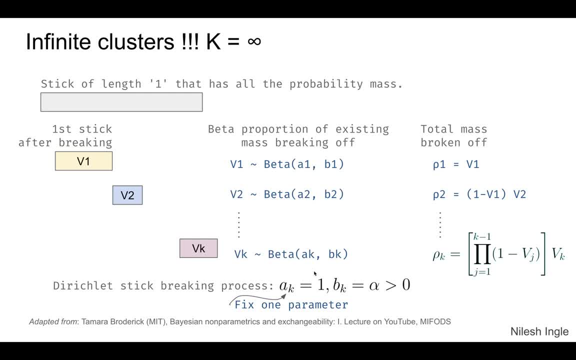 and all the a's could be set to 1, and all the b's could be set to a value that is greater than 0, and then, so that that would be the way, so the analogy of breaking the stick would continue to be the same. so that's in essence that it is the direct list. 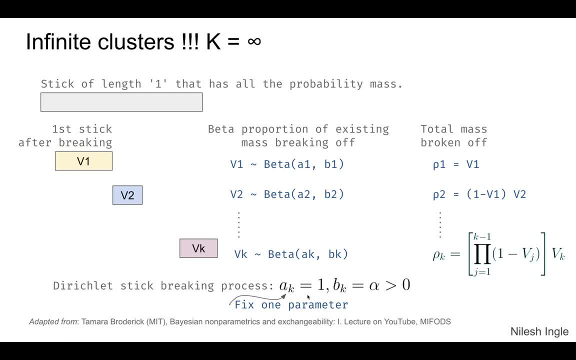 stick breaking process, where we are fixing one parameter and again, as we saw in the previous style, speaking without KIRBY definition, and we can now think that let's knew this data and again it's only the norm that it's either 0 or 0, and to apply this regulation, we can define with 0 as 0 and between 0 and minus 1.. So to apply this regulation, we need to define a moveset with few values and if eq 0 only, we are going to write. and then so that that would be the way it's, so the analogy of breaking the stick would continue to be the same. so that's, in essence, the dirichless stickaram. we are fixing one parameter and it has, in essence, we have fly in between 1 take and a little bit more of a Women's law proposalуп. 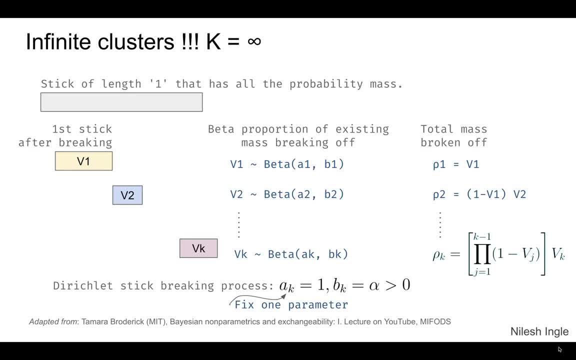 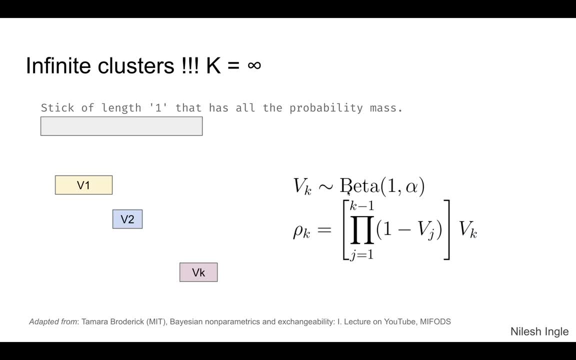 and again, as we saw in this case. here is the mathematical notation. so we have VK. that comes from beta, distribution of 1 and alpha. we set all the A's to 1 and we are saying that all the B's would be a value of alpha. that 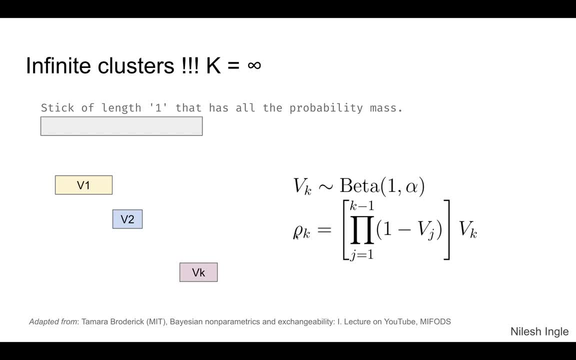 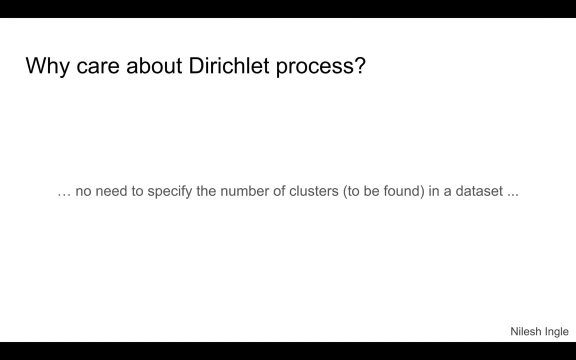 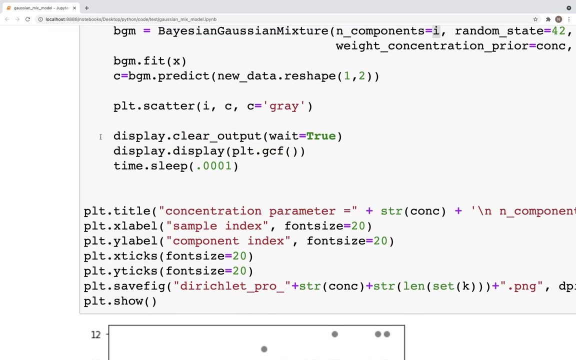 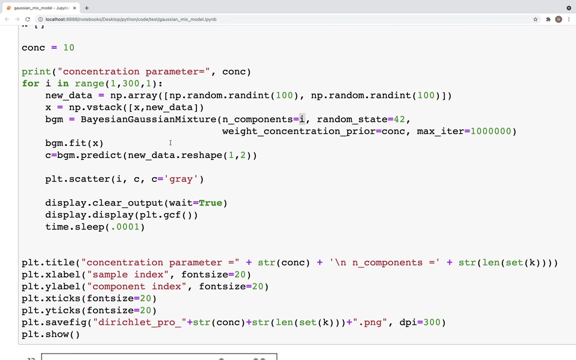 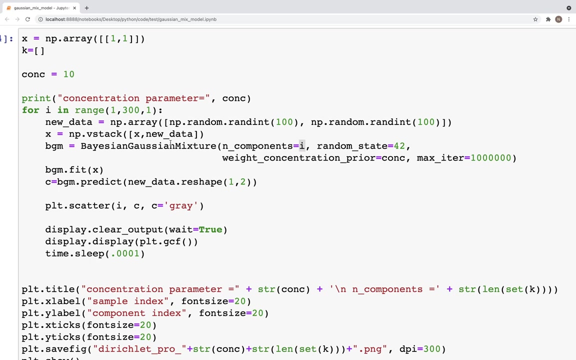 is greater than 0, and then we can. we can get the values for Rho K, which would be product of the relation that's shown here. now let's look at the Dirichlet process in action. so here you look for Rho and here it looks like we have very much. 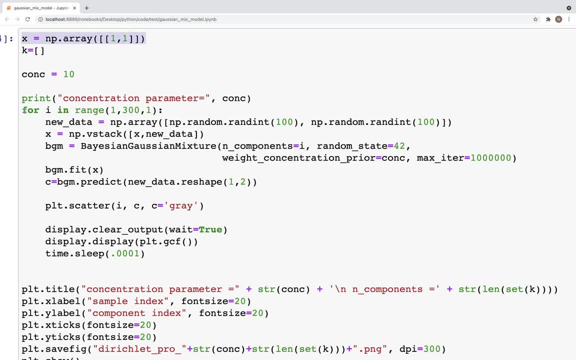 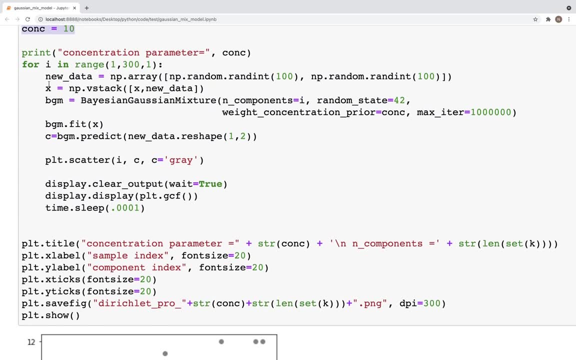 data point. even before this is done. so let me, Joseph, quote up in Jupyter notebook: what I'm doing is initializing this data point X, 2, 1, 1, and then within this for loop, I'm setting the concentration parameter through ten and within here I'm creating a new data point and we'll be iterating for 300 times and using the bayesian gaussian. 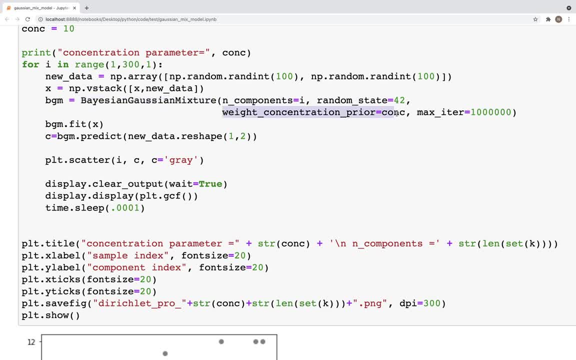 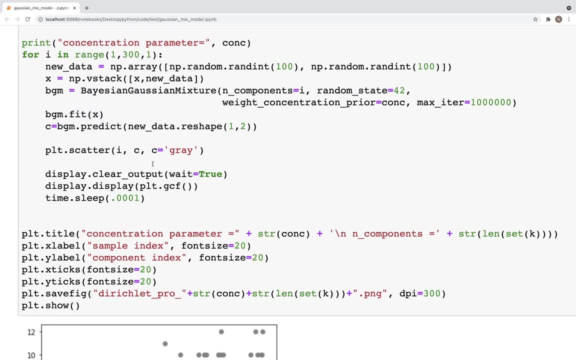 mixture with where we can input the concentration parameter fitted on x and then predict the value. and we are trying to predict the class, and what i'm trying to do is plot this class as it is predicted for each of these new data points. so what? what i want to show is, if you 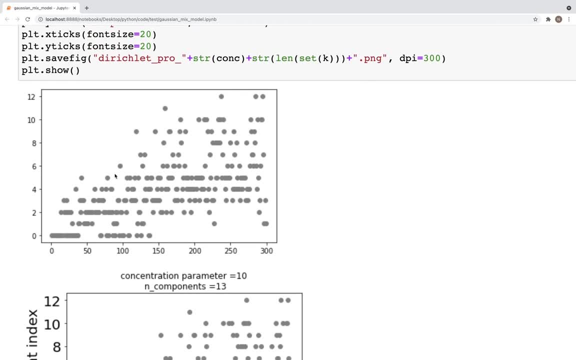 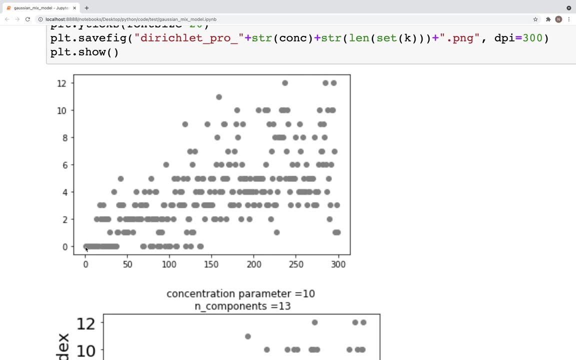 look at this particular plot here. we'll look at the animation shortly, but before we do that, what happens is, as the very first point when we begin the process, the very first iteration, all the clusters would be empty. so when a new data point comes in, it gets assigned to, let's say, cluster one. so these are the cluster. 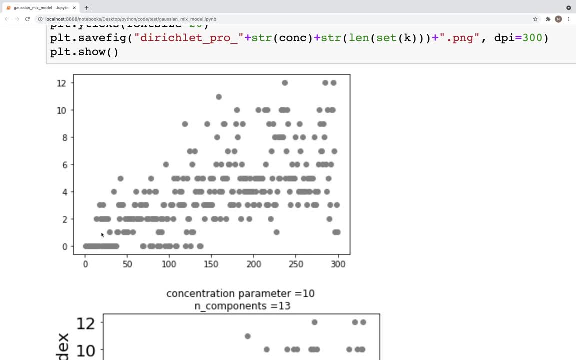 numbers, so cluster. there are 12 clusters right here, so cluster one. then after that a second data point comes in, so that data point can now be either assigned to cluster one that already exists or it could be assigned to a new cluster two that could be in which there is no data point yet. similarly, if a third data point comes in now, it could be assigned. 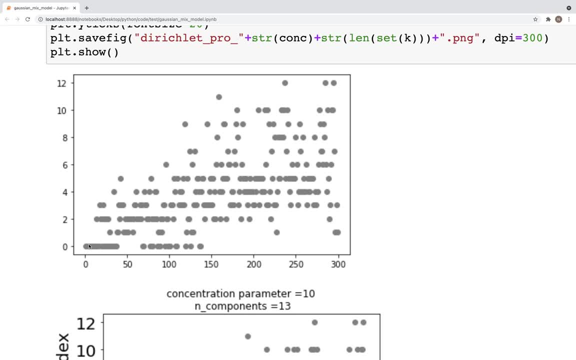 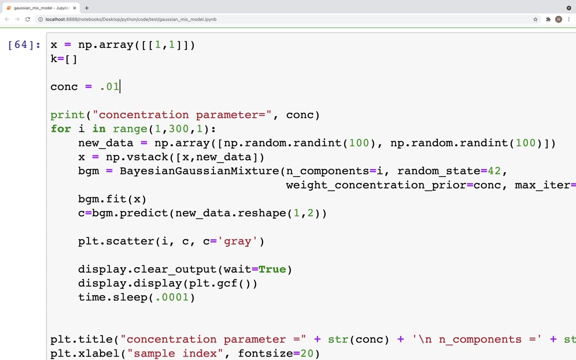 to cluster one, or it could be assigned to cluster two, or it could be assigned to a new cluster three, and so on. the process continues to repeat, and that's what i'm trying to show here. so let's run this. so here we first have, we can try to set the concentration parameter, let's say 0.0001. 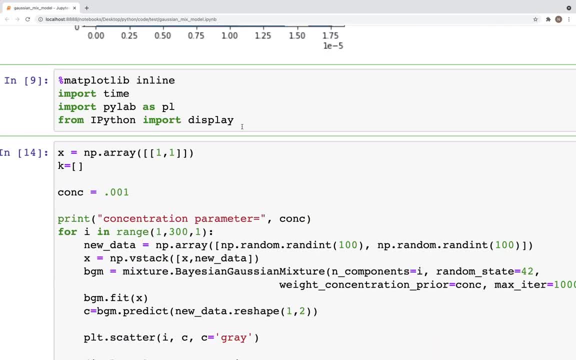 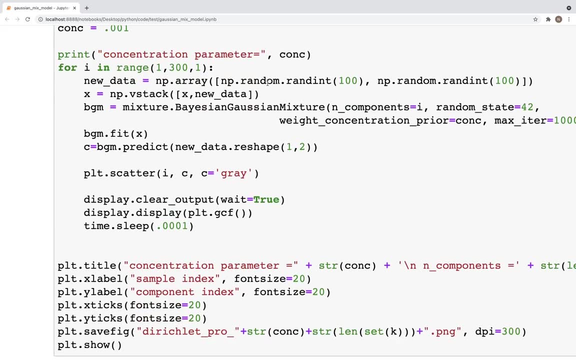 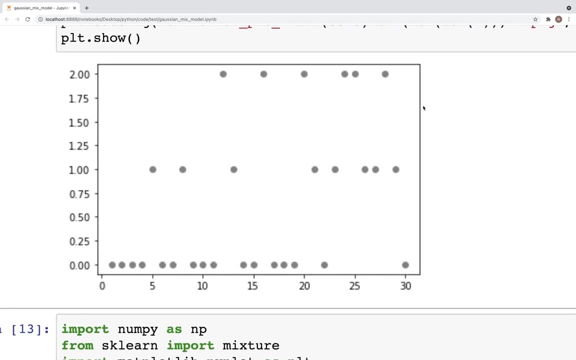 and run this. i'm going to run those libraries and let's run this now. so this is how we can see, as the new data points are coming in, they are getting us, and right now we have just three clusters. one is labeled, one at zero, one and two so with the value. 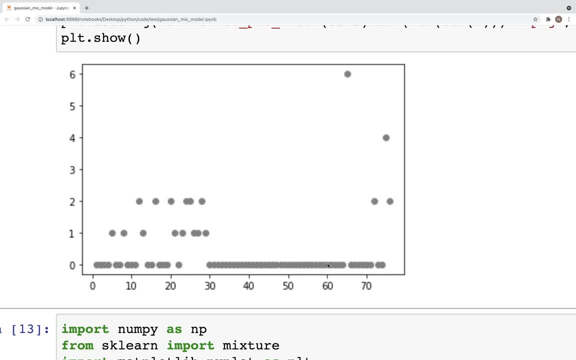 of the input hyper parameters set to very low number. we see that most of the values are put into the cluster 0. as we can see by this line, there are some, well, some- data points going to clusters, other clusters. so we now have a total of six clusters that are created and we still have 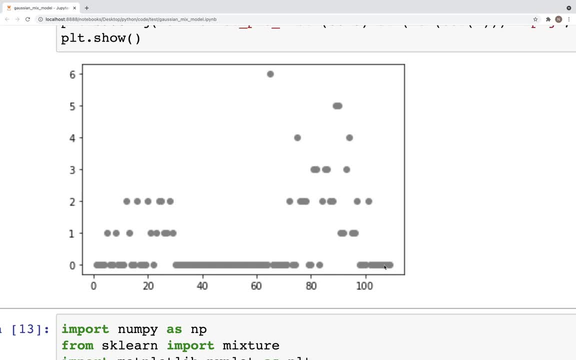 200 more data points to go. so this process would continue and we may be able to see a few more data points and joining the cluster one. so if you look at this dirichlet process, if you read about it more, the the general idea is that if there are clusters that already have data points in them, the chance that a new 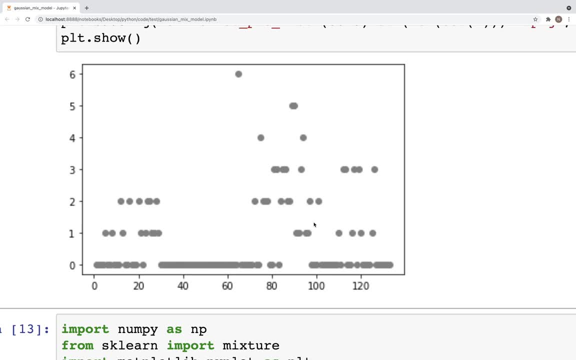 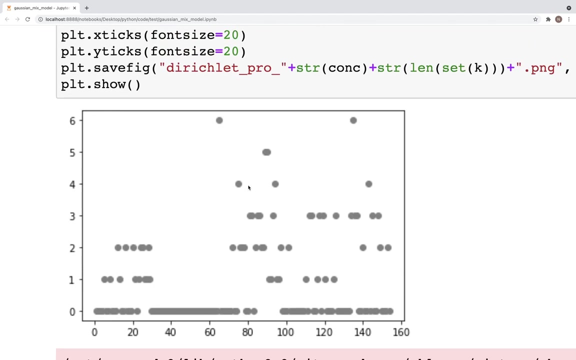 data point would come in, get assigned to an. a data point that has data, already has some data points, is more than getting assigned to an empty cluster. so i'm going to stop this run right here and we'll look at. we'll update the values for the hyper parameter and run this again. 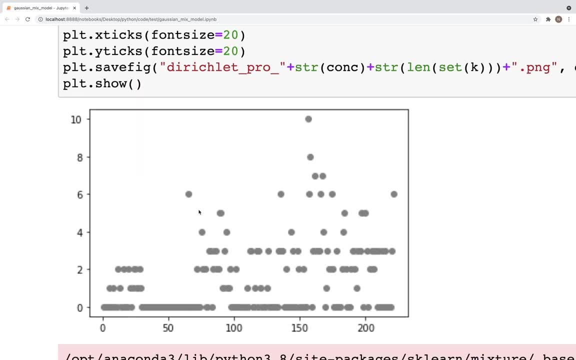 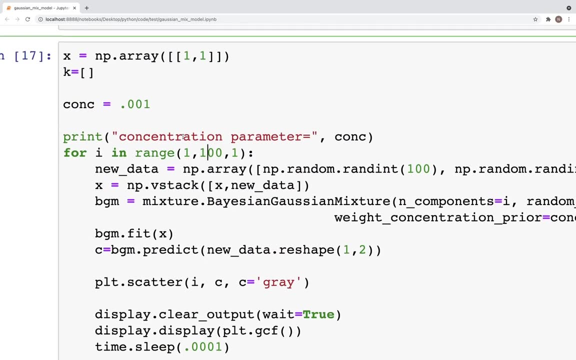 maybe set this to just 100. okay, i've stopped this now and let's go back up. i'm going to change this to 100 iterations and let's change the concentration to one and see what we get. so why don't we do this? uh, i'll keep this as 0.001 and copy this entire thing. 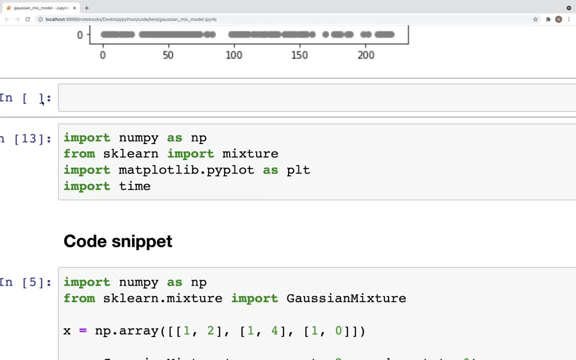 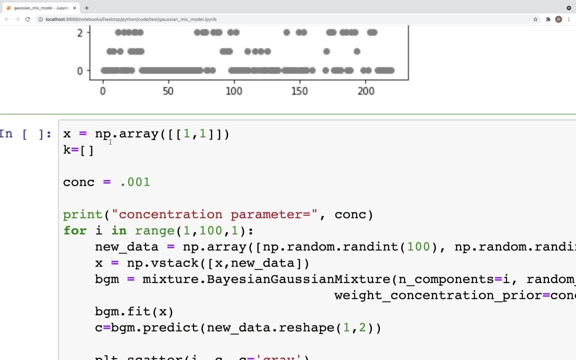 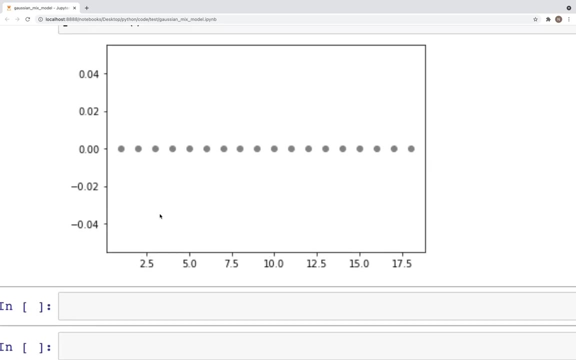 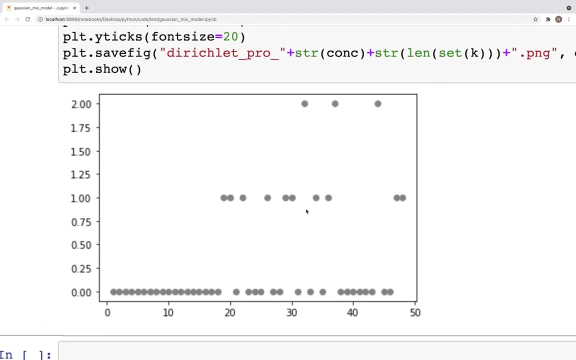 and then paste it down here and we create more cells and the idea is to then compare how are different they are. so we'll put that as one and run this so with one. uh, as we can see, the way these data points are getting assigned is a little different than. 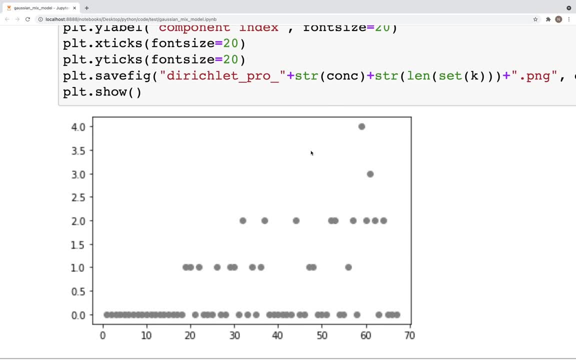 what we had with the value for uh 0.001, and here we can see that uh- still the cluster 0 has more data points. but then we just have four clusters so far and we have more data points going into the newly formed cluster 1 and the cluster 2. 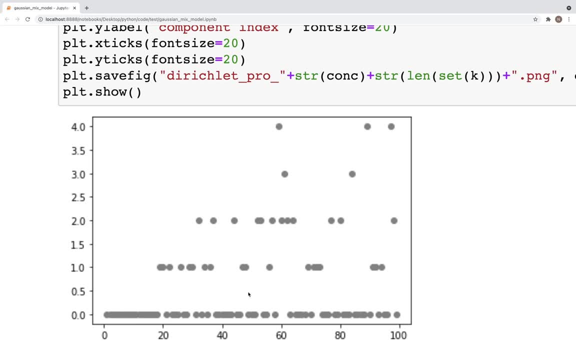 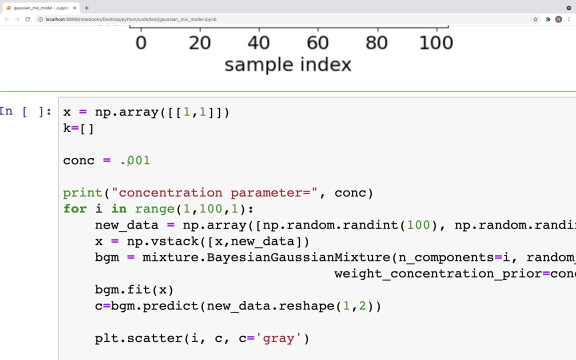 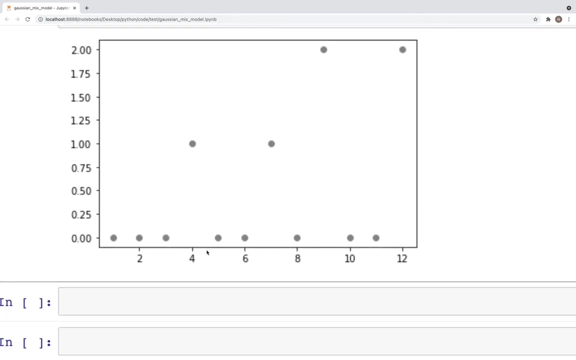 and here, as compared to beta distribution, we didn't expect that this would be a uniform distribution and accordingly we do still see higher number of data points assigned to the cluster one. next, let's add another layer to this and run this with a concentration value for 10.. so with 10, 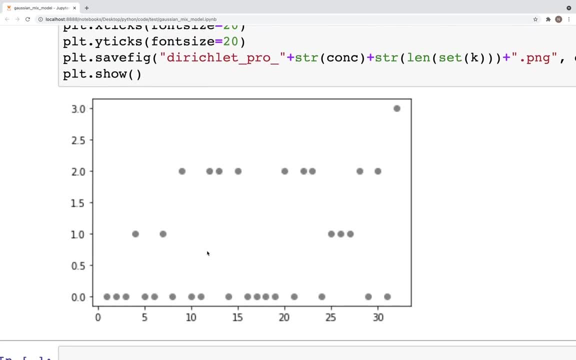 we can see that the data points are getting assigned to the cluster 1, and now what we are trying to do is we are moving towards, uh, equal, assigning equal weight to the data points, uh, but, as we can see, they are still getting randomly assigned to all these clusters. we. 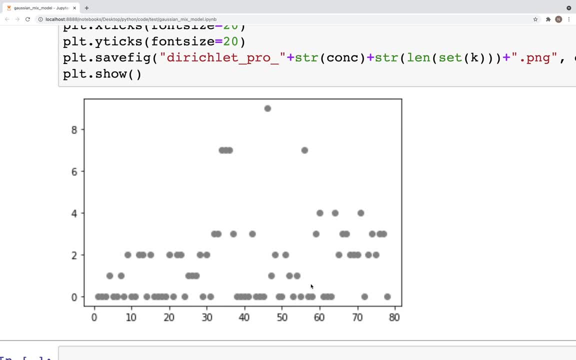 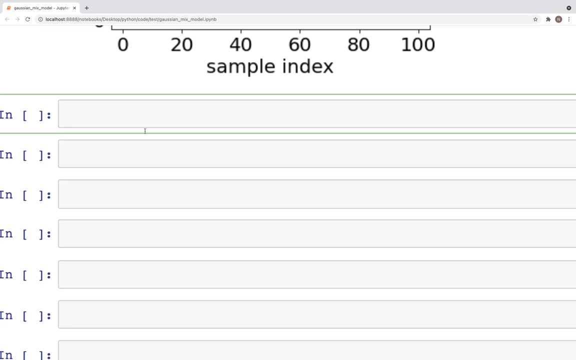 we have um eight clusters so far, maybe nine clusters, and you can see, in this case, maybe little less data points were assigned to cluster zero as compared to the other clusters. so that's the hundred, so okay, so that's, it are 10. and now let's try a very high value. so let's try one. 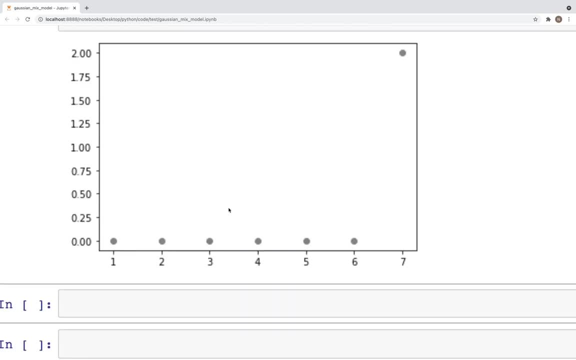 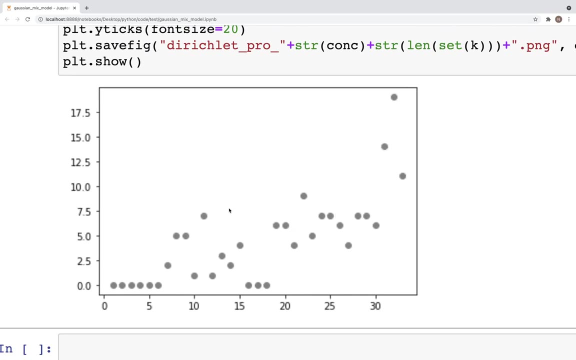 maybe 10 000, and in this case the values are, they are. they look different. as you can see, you, it is become very easy to create more cluster. so we have already reached a 20 separate clusters, or 35, and we can see the big difference that. 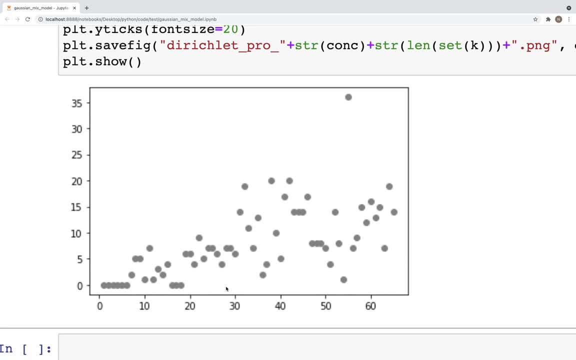 the tendency is to assign an incoming new data point to an empty cluster rather than assigning it to a cluster that already has some data points. so the cluster 0 has very few data points in this particular scenario, where the value of hyper parameter is much higher, and we've already reached 40 plus clusters and we can see this increasing trend. 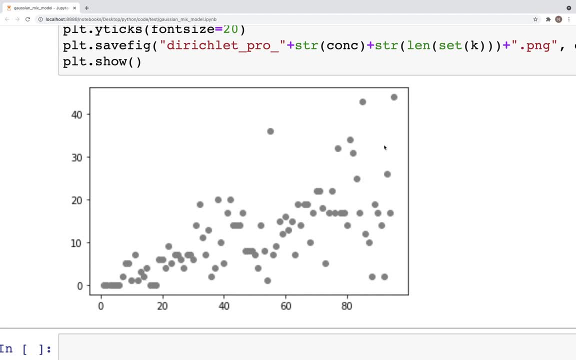 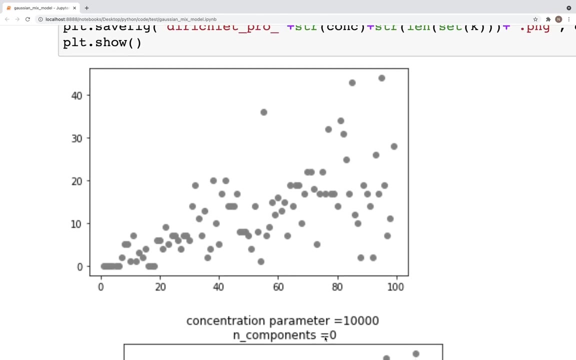 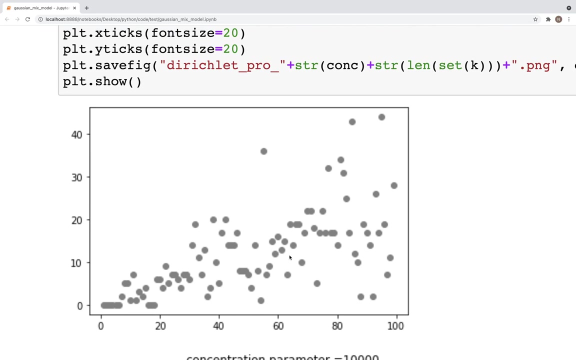 as the Dirichlet process continues, and now, by the time we reached 100, we are close to maybe 45, 48 uh clusters. so that's this is wrong here. n components is not zero. so that's the whole idea behind the Dirichlet process. as you can see, with higher values of hyper parameters, this is a 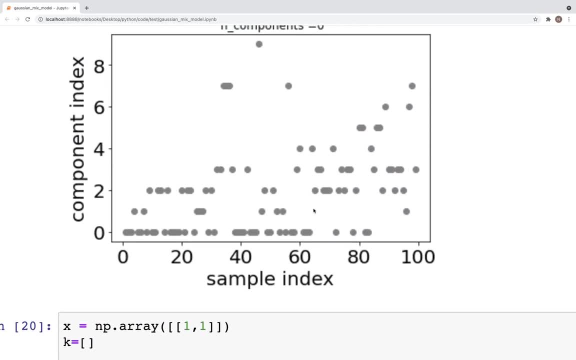 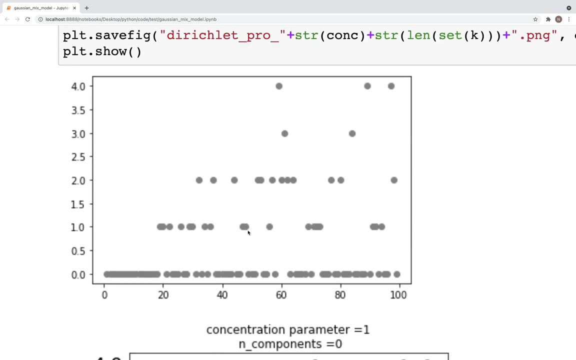 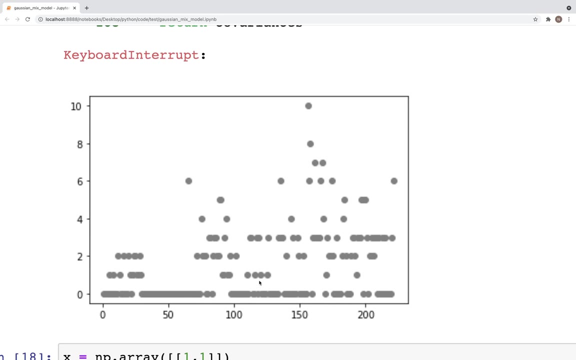 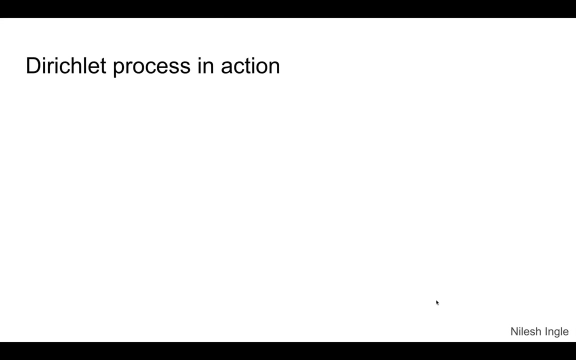 the data is generated. as we go on, go on reducing the value of hyperparameters, as we can see down here, we start putting more and more emphasis on one of the clusters. now let's get back into the powerpoint slides, and here the question that we can ask is: why do we care about the Dirichlet? 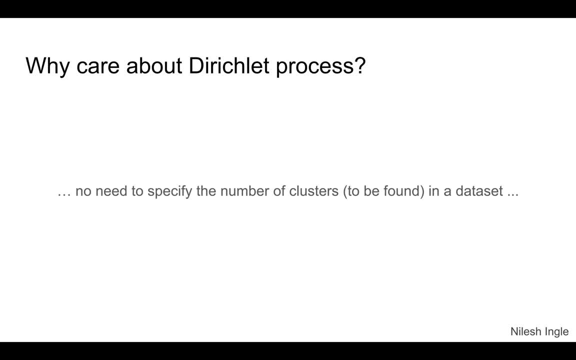 process and the reason is we do not need to specify the number of clusters ahead of time to be found in a data set. so this could be useful in instances where we cannot visualize the data and even if we are able to visualize, the structure of the data is such that we cannot identify. 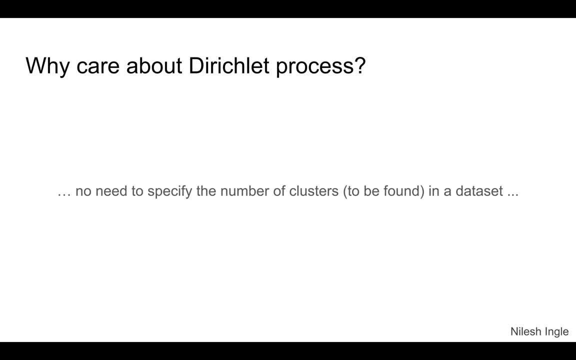 any clusters visually in the data set to set the value of k. so the Dirichlet process could help in this way in those instances where it is able to find the optimal number of clusters. now, what is variational inference and why are we using it? so, as we looked earlier, 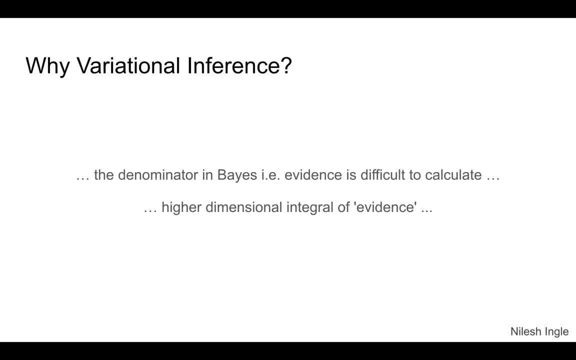 in when we are trying to estimate the posterior based on the likelihood and prior, the denominator, which is the evidence, can become difficult to calculate, even for the computers, and so there is alternative way to find the value for the posterior, and that's where the variational inference comes in. 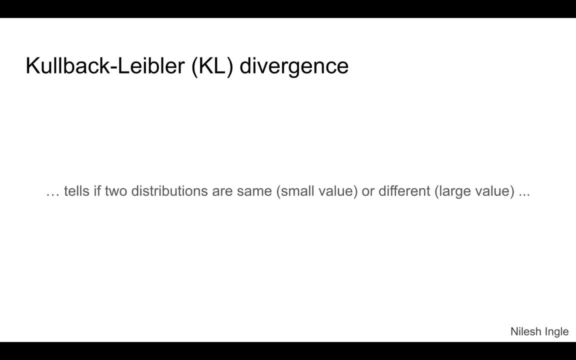 the methods within the variational inference coming, and that's where the kl diverge. kl divergence is also used, as we discussed earlier, which is cullback libular divergence, and it tells us how similar or how different the two distributions are. so lower the value. the similar those two distributions are, farther the 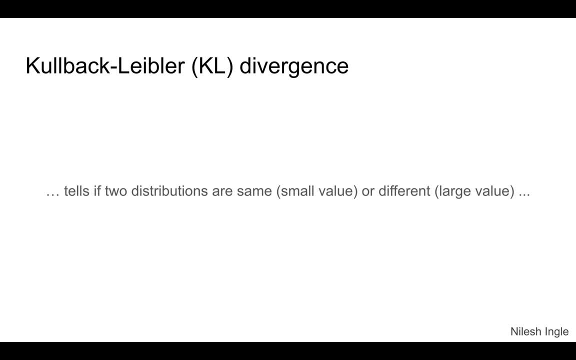 value, the different they are, and that's used to gauge the iterations. when we are trying to optimize now, random initialization is needed in these methods and initialization can affect what the final results would be. so the general idea is to run initial. maybe k means to get a general idea on the cost. 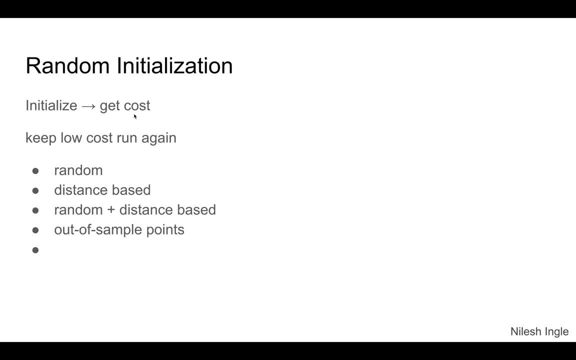 associated with the initialization and the cost associated with the initialization, with that type of initialization, and then find the values for seeds that give the lowest cost and then use that in the next steps. and then these could be of different types, random, distance based or both, or those could be out of sample points. now how do we know if? 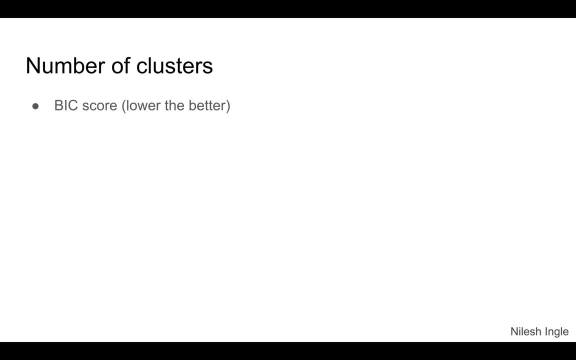 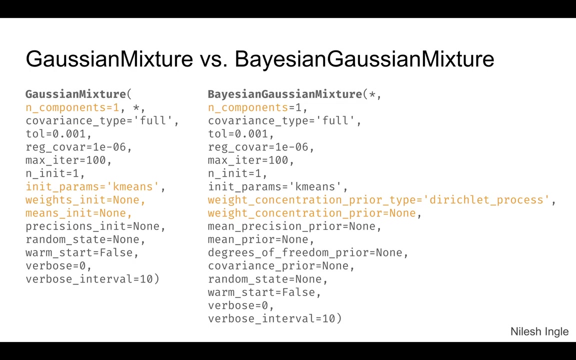 the number of clusters that we have found is good or bad or is it optimal. so that could be to help kind of approximate that we can use the BIC score. so the lower the score the better, so the better it is. and finally we have the comparison between the two methods that are: 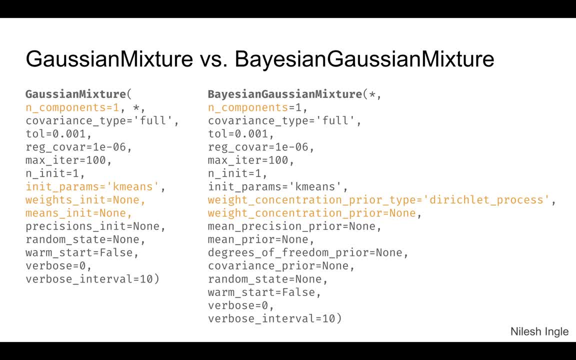 available in scikit-learn and the other methods that are available in scikit-learn and the other methods that are available in scikit-learn Gaussian mixture and the Bayesian Gaussian mixture. so the Bayesian Gaussian mixture uses the variational inference, the Dirichlet process, that we discussed in the latter part of this. 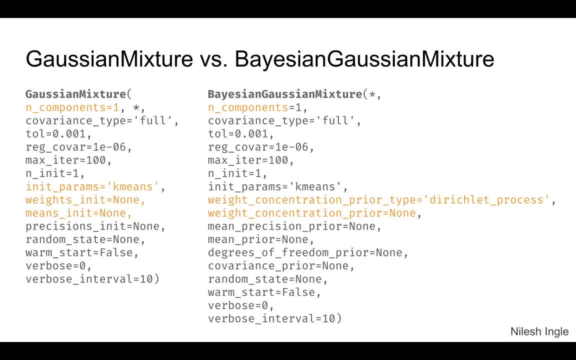 series of videos and the initial part where we talked more about the k means is what the Gaussian mixture uses. so in Bayesian Gaussian mixture, points to note is that the Bayesian Gaussian mixture points to note is the factor characteristics of the normal distribution is the respect you can use a. 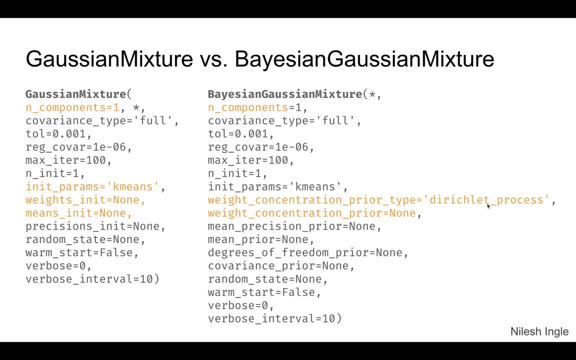 or an arrow. here自 têm certificate, a factor shouted obvious or false? this who says that we can specify the weight concentration prior type, which is that we can specify the weight concentration prior type, which is the Dirichlet process by default, and we can question classified the values for. 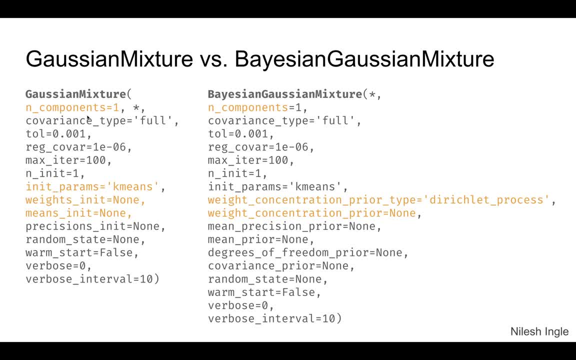 the few. these的是 contraries for the V concentration, which is known by the follow and we can alsoところ w and you can set the value for tolerance. so in and you can alsoところ w starting in the state breaking process is to be useda of the 있点 folkヾ. 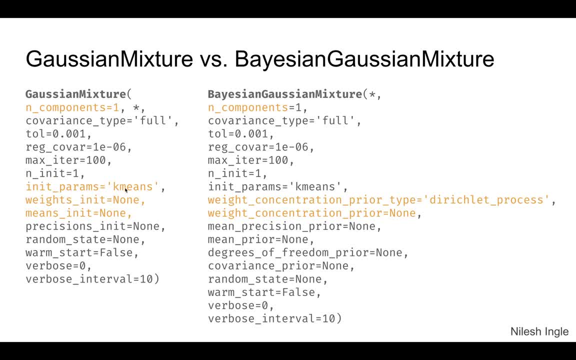 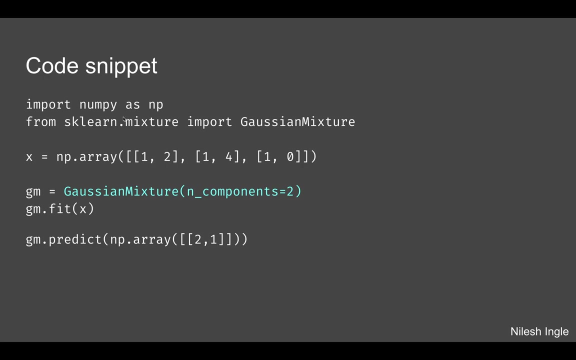 then we have initial parameters- uh can be found by k means- and then we have the initial weights and initial means, and again, this also has the initial parameters that can be defined by k means, as it's just not highlighted in orange. the code snippet is straight simple. we have the library sklearnmixture.